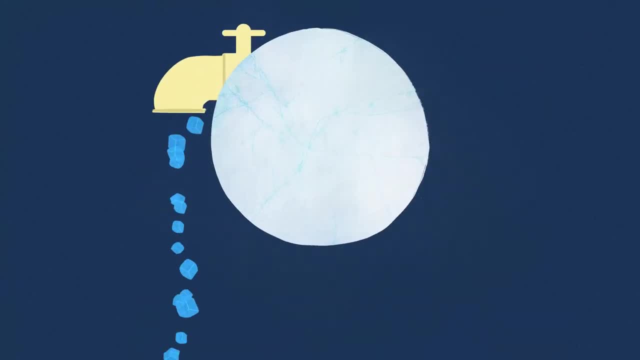 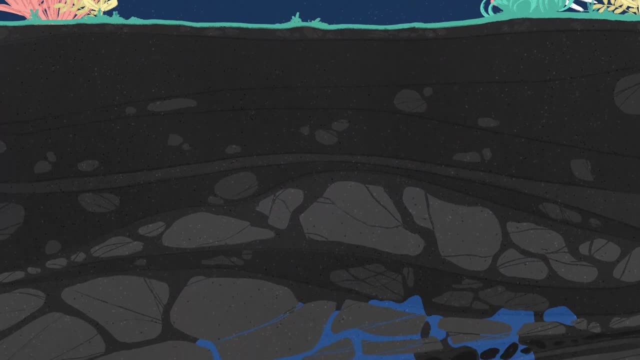 making it pretty tough to access as usable water. The next most abundant source of fresh water is what's known as groundwater. As water seeps into the ground from above, it fills the cracks, pores and spaces between bits of rock, If you look deep enough. 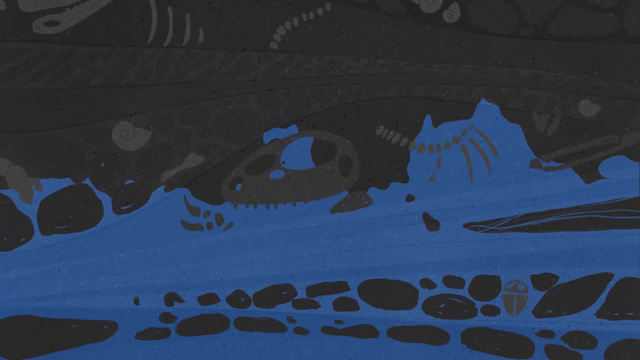 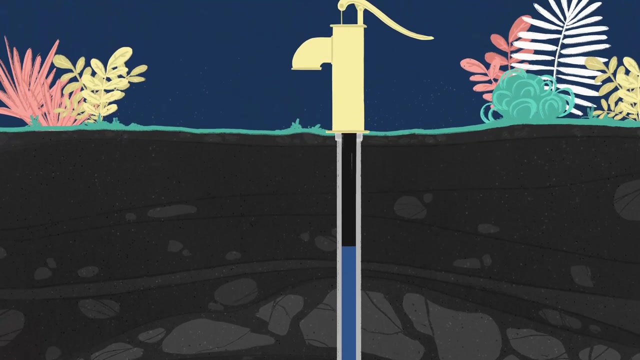 you might find that all the space between rock particles has been filled, forming an aquifer. Aquifers store huge amounts of water that can be pumped out to the surface for drinking water and irrigating crops. Like a savings account, it can take a long time. 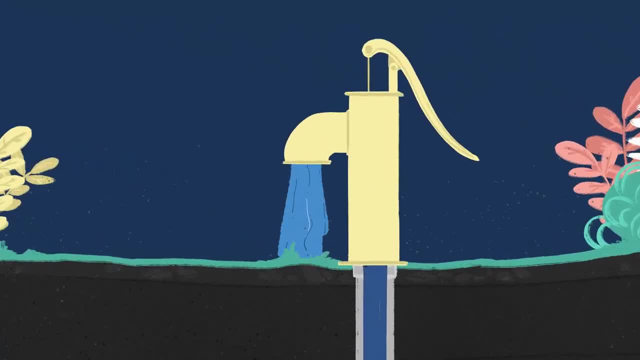 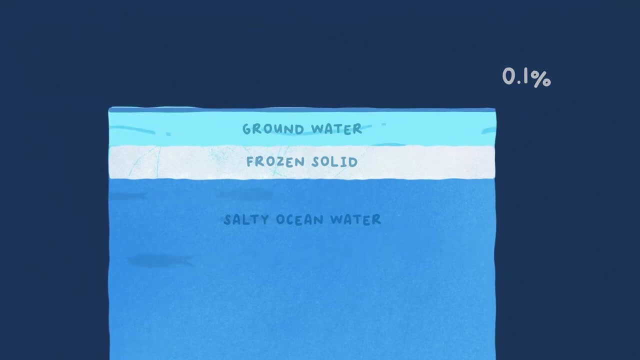 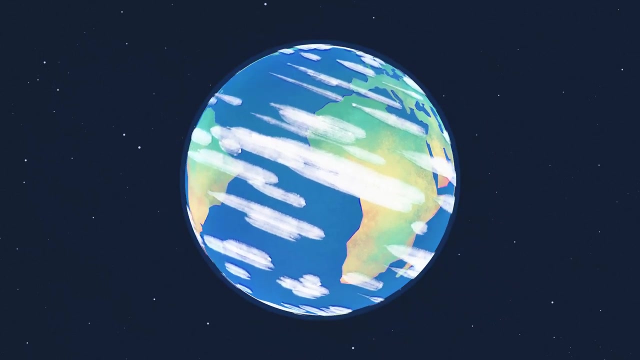 even centuries for groundwater to accumulate. That leaves just 0.1 percent of all water that isn't salty ocean water or freshwater that's frozen or buried in the ground. If you are looking for easy access to what remains, think again. Most of this tiny fraction of Earth's water is frozen as permafrost. 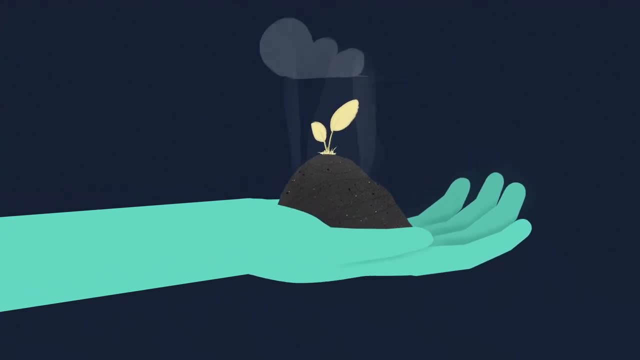 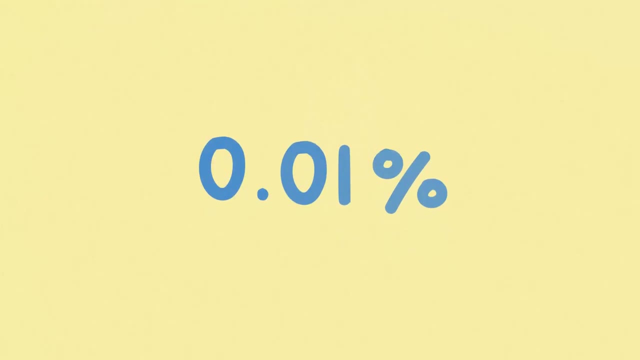 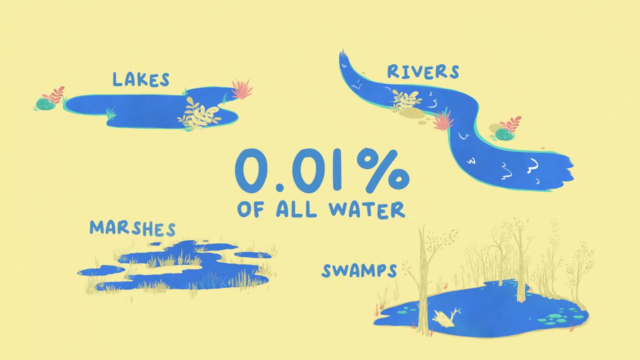 some exists as moisture in the soil, a bit is in the atmosphere as water vapor, and some makes up the water that exists within living creatures. Just 0.01 percent of all water on Earth is on the surface, in lakes, rivers, swamps and marshes. 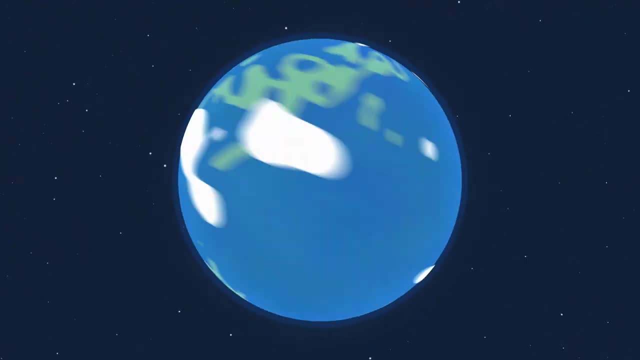 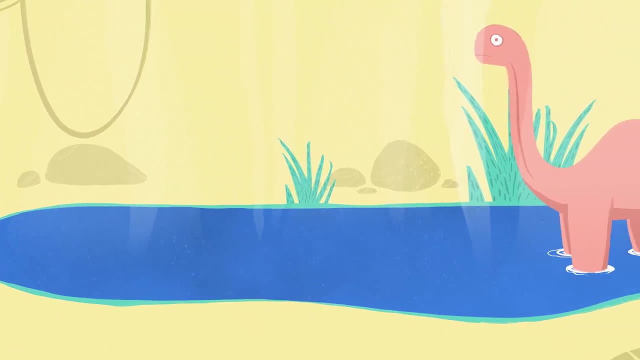 Most water on Earth has been here for billions of years, and during that time any single drop might have moved between different parts of Earth's water budget. Moving from one part of the budget to another, a process known as the water cycle- can happen quickly. 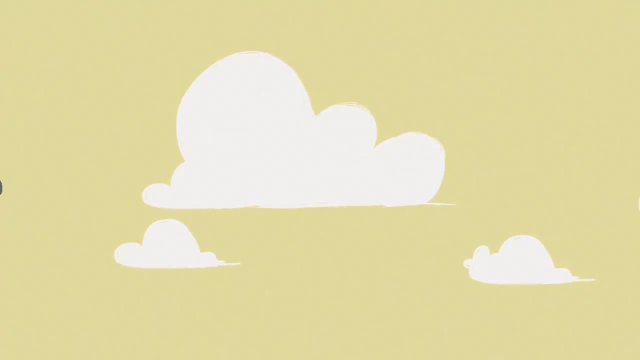 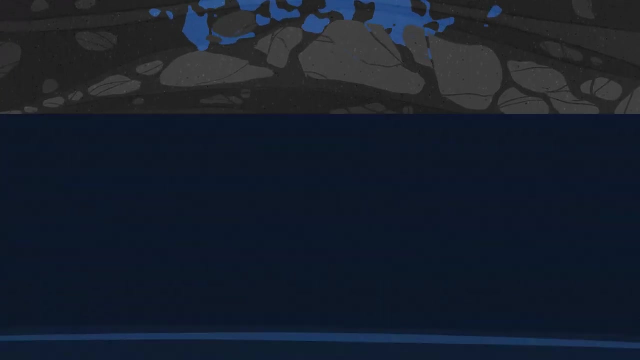 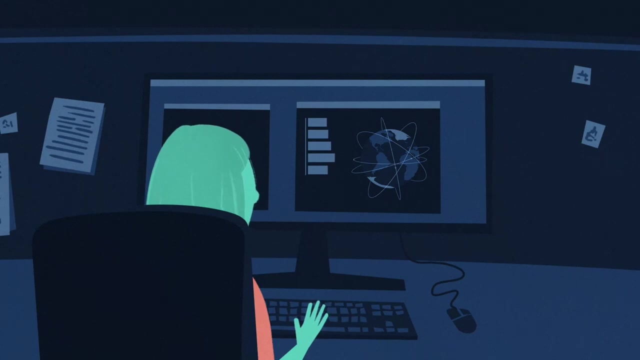 like when water evaporates from a lake and moves to the atmosphere. It can also happen slowly, like when water makes its way deep underground. Understanding where these different forms of water exist and how they move is an important part of understanding our planet and planning for future water needs. 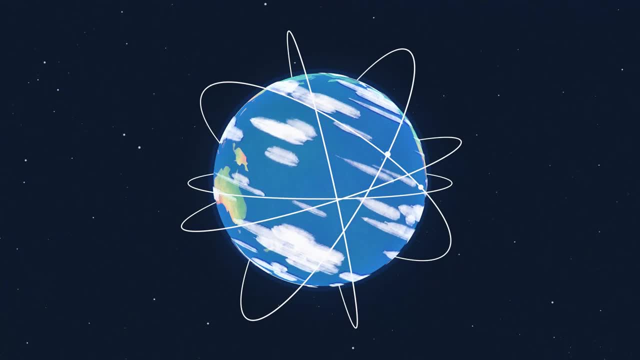 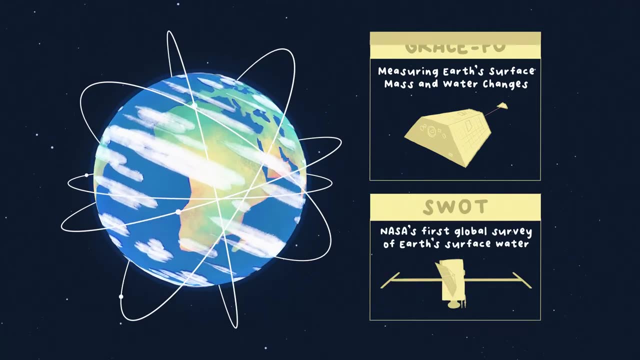 NASA has a fleet of satellites studying the location and movement of Earth's water, each designed to measure certain types of water. Some measure the movement of groundwater or ocean currents, while new missions like SWAT and NISAR will also fill gaps in our knowledge by measuring freshwater and possible hazards. 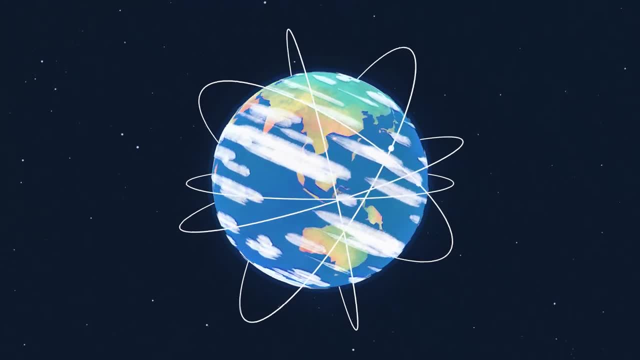 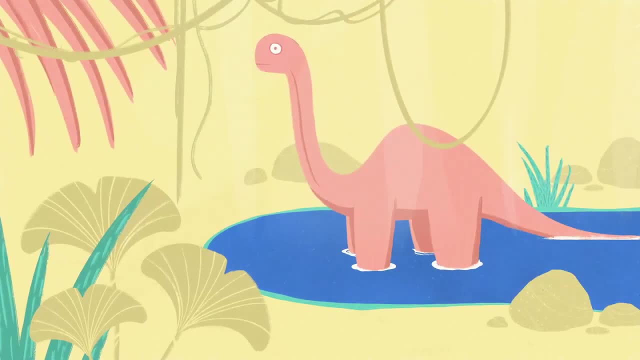 Together. these missions help bring NASA's water budget and cycle into focus. So next time you feel a drop of rain on your face, imagine all the places that water might have been during the last few billion years and where it might be in the next.